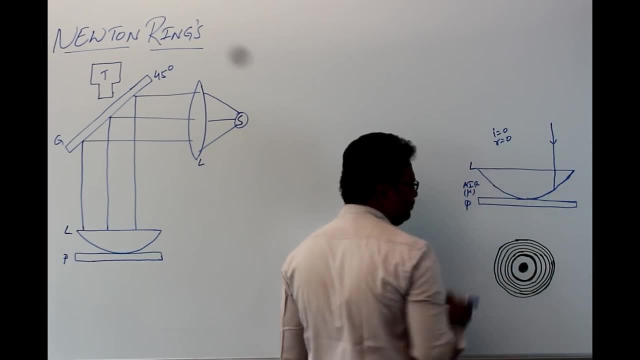 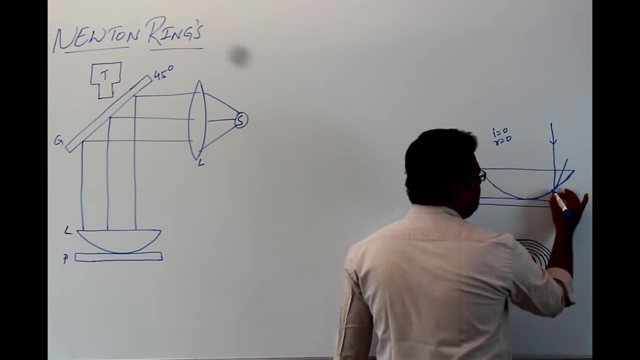 by air of refractive index mu. Now, at the top of the thin film, some part of light ray will reflect and some part light ray will refract. And again from the bottom of the thin film the light ray will reflect and moves out. 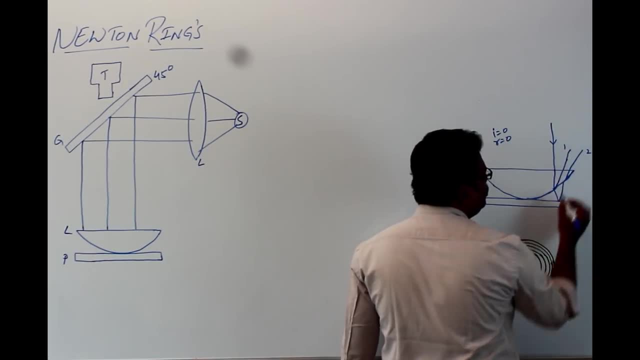 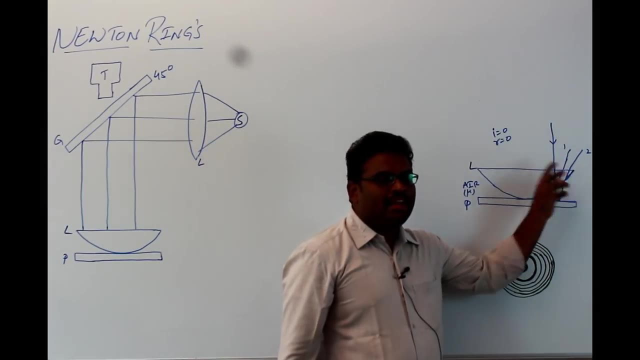 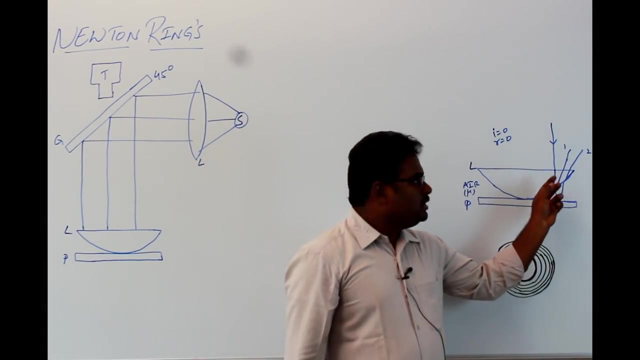 Since the light ray 1 and 2 are in a position to get superimposed. So, due to that, if the path difference between the two light rays is n- lambda, then you will get a dark fringe- sorry, bright fringe. and if it is n plus 1 by 2 lambda, we will get a dark fringe. So 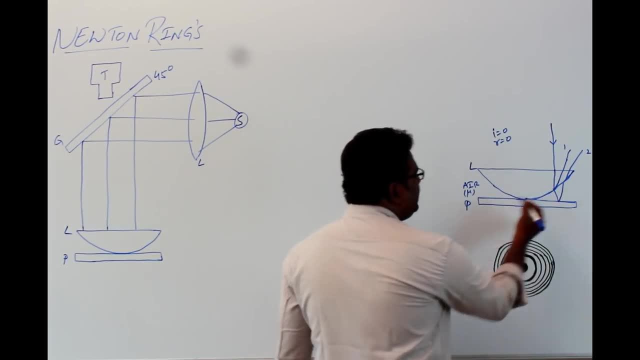 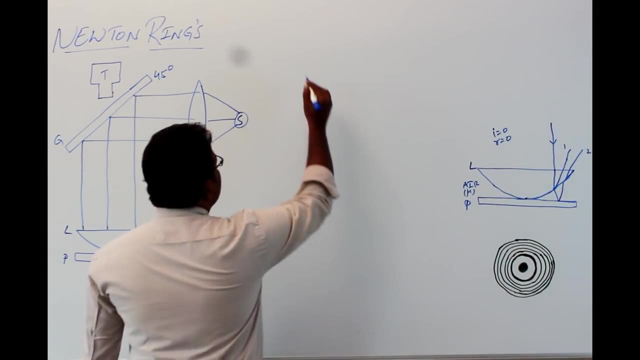 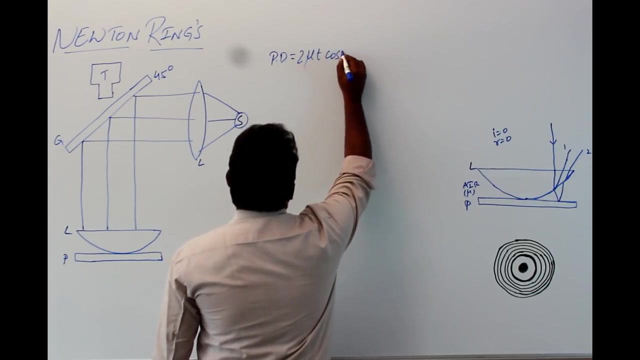 if you consider the path are already we calculated the path difference between the two light rays which are reflecting from a thin film. So the path difference between the two light rays which are reflecting from a thin film is 2, mu, t, cos, r plus r minus lambda by 2, where 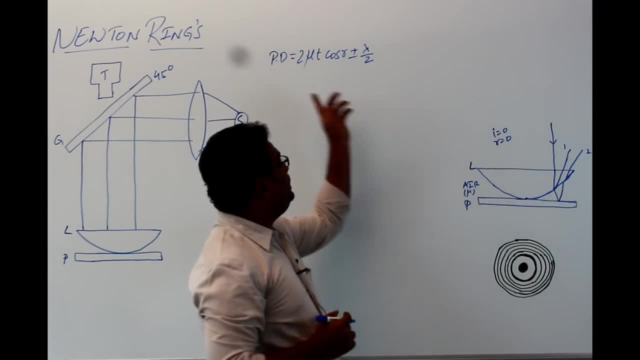 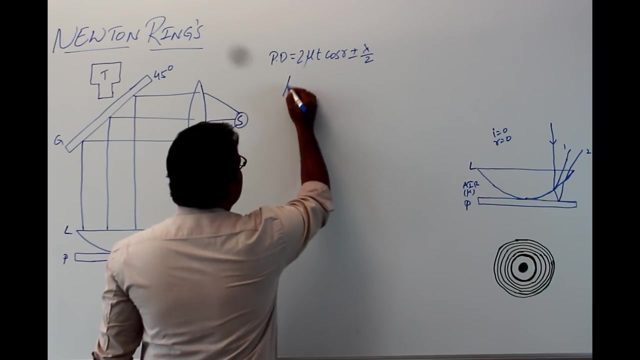 mu is the refractive index of the thin film, t is the thickness of the thin film, r is the angle of refraction, which is 0, and lambda by 2 is the wavelength that we are using. And now for this particular Newton's rings experiment: the thin film is formed by 8 that. 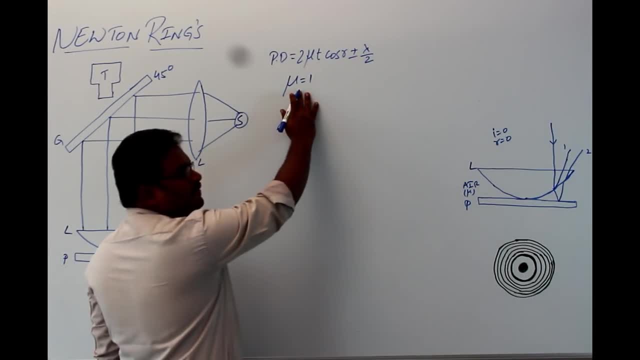 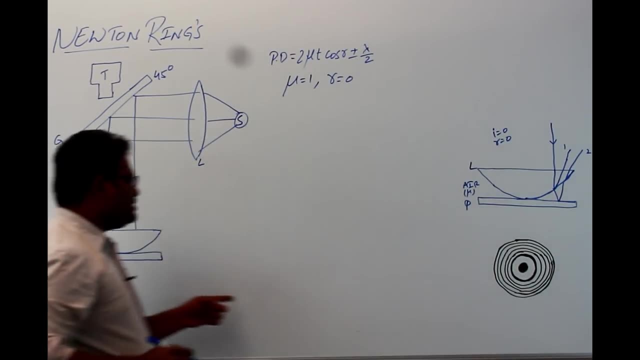 is why mu is equals to 1.. So refractive index of 8 is 1 and angle of refraction are also 0, because this is a normal incidence, Since light rays are incidenting on a plano convex lens normally. So whenever light rays are incidenting like this, the same will reflect. 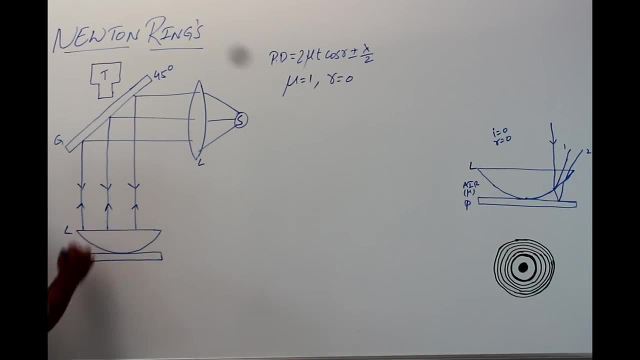 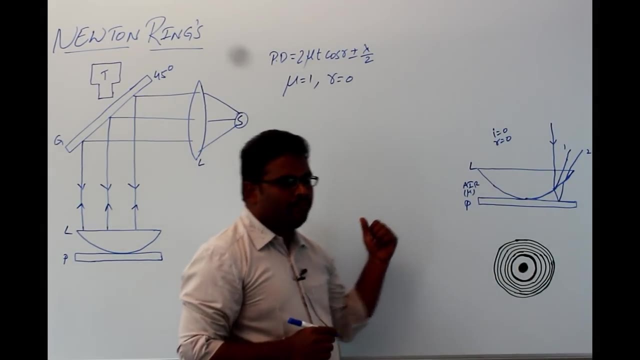 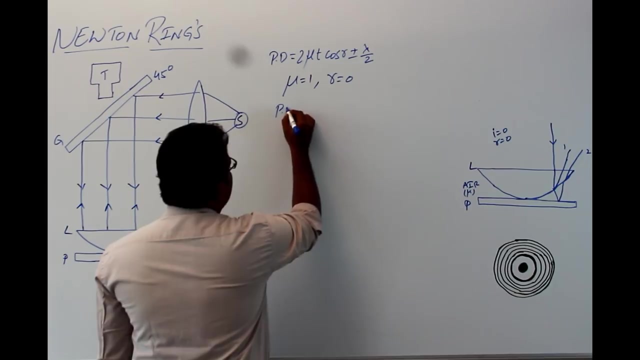 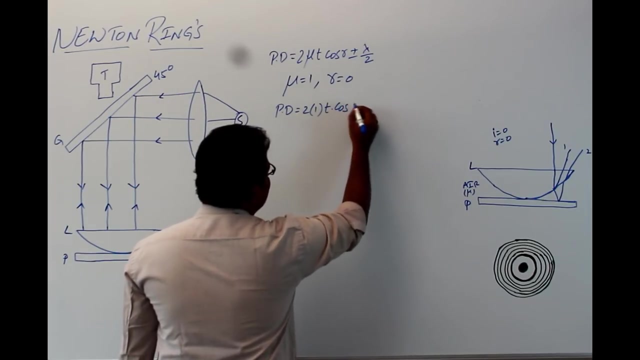 back and both get superimposed and you are getting alternate to bright and dark range. Why the centre of Newton's rings is dark and reflected case that we are going to see now, Now. so now the path difference will become 2. mu is 1, t cos r is 0 degrees plus or minus. 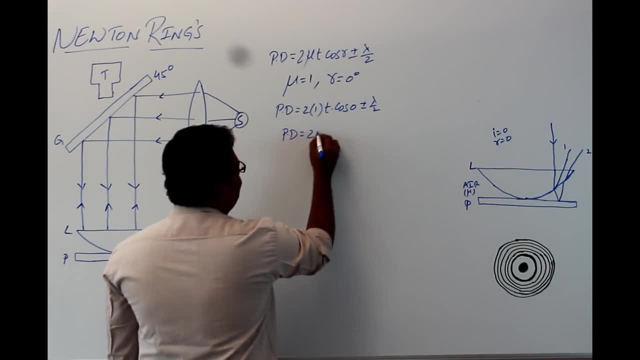 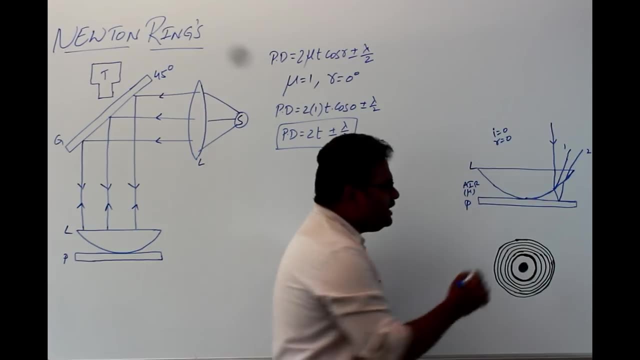 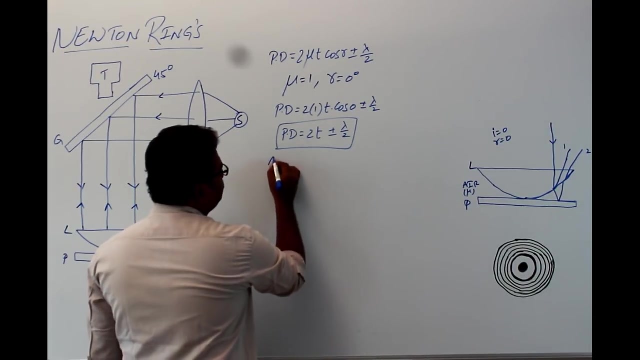 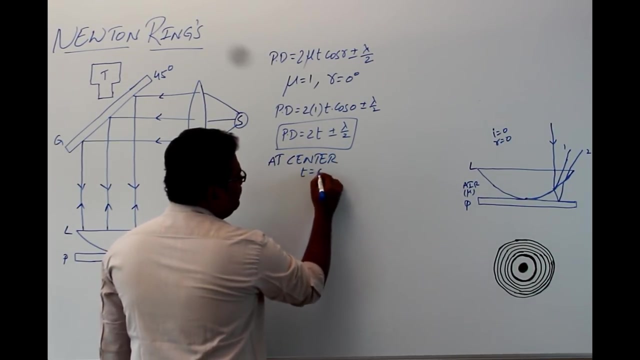 lambda by 2.. So now your path difference will become 2 t plus or minus lambda by 2.. This is the path difference between the two light rays which are reflecting from the thin film in Newton's rings. Okay, Newton's rings experiment. So at the centre the thickness of air film is 0.. At this position, 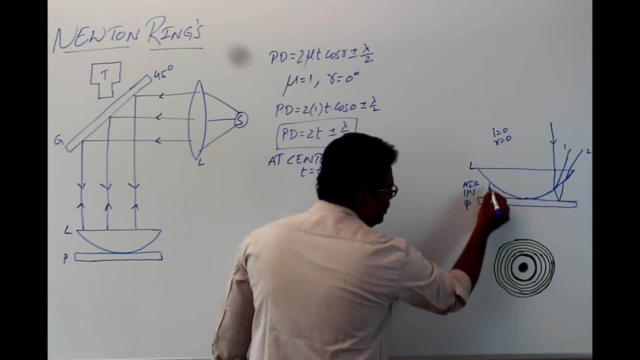 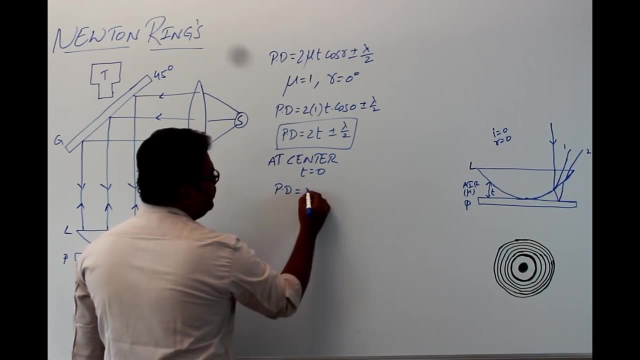 the thickness of air film is 0, and here you can have some t, But at centre the thickness of the air film is 0. That is why your path difference now will become 2 of 0 plus r, minus lambda by 2, and path difference is equals to lambda by 2.. 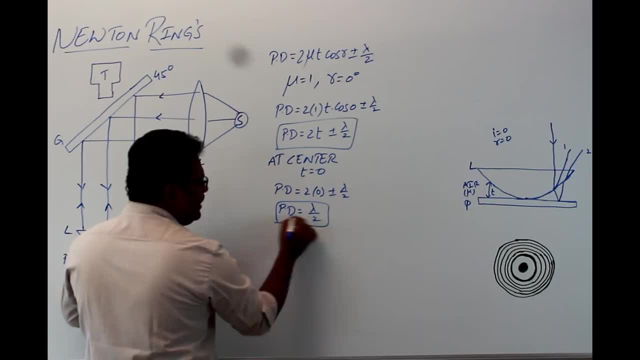 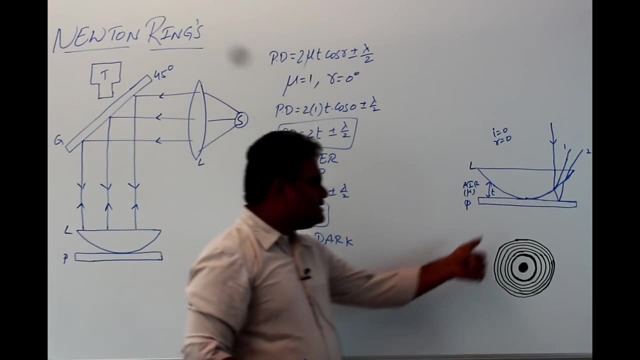 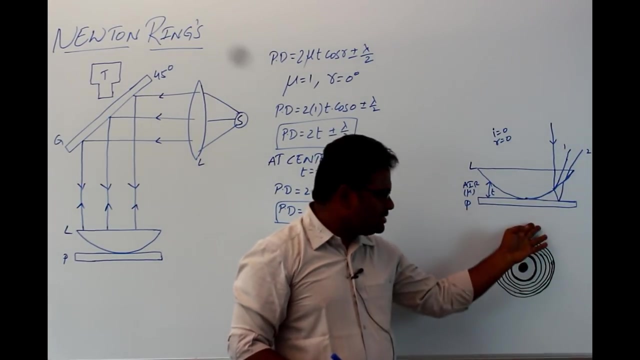 So if it is, if path difference is lambda by 2, one can have a dark fringe. That is why the centre of Newton's rings experiment, the centre of this one in reflected case, not in transmitted case- in reflected case is a dark one, and after that we have a we. 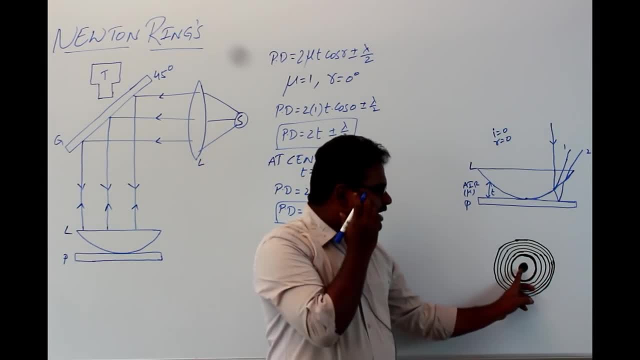 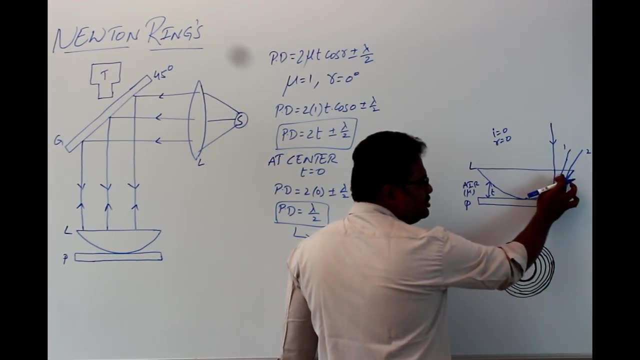 are having a bright and alternate to bright and dark rings. Why we are getting alternate to bright and dark rings is Since, suppose, at this particular distance, if the two light rays are superimposing and their path difference is a lambda. in this position you can see a white fringe, Suppose. 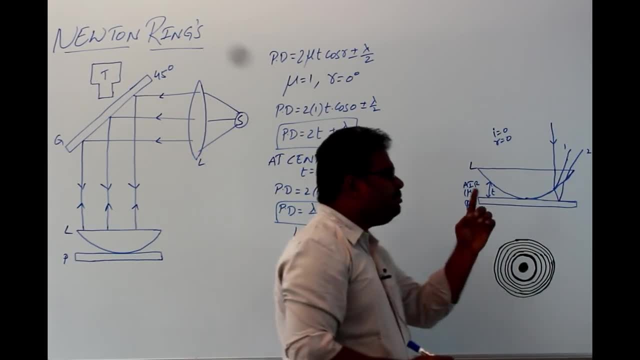 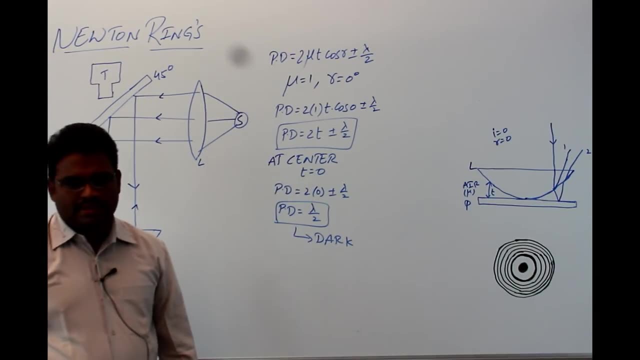 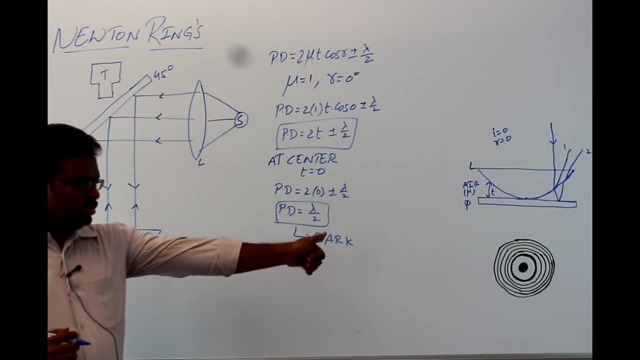 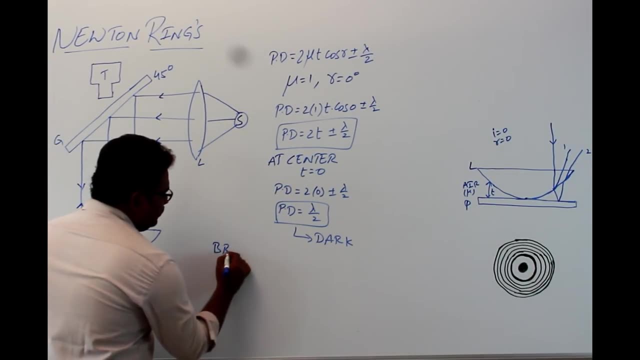 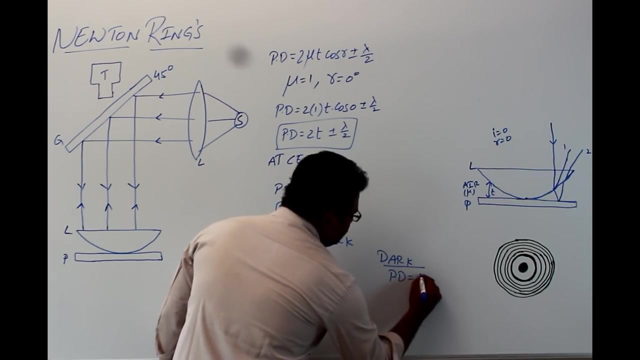 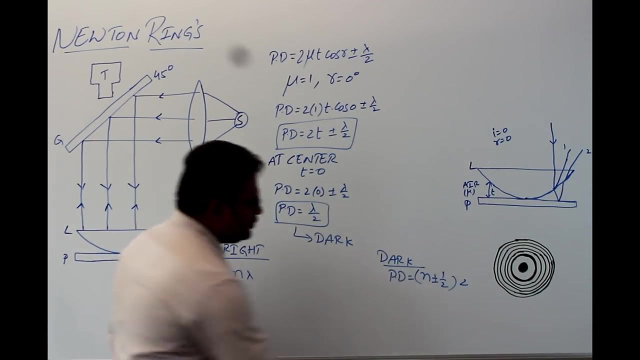 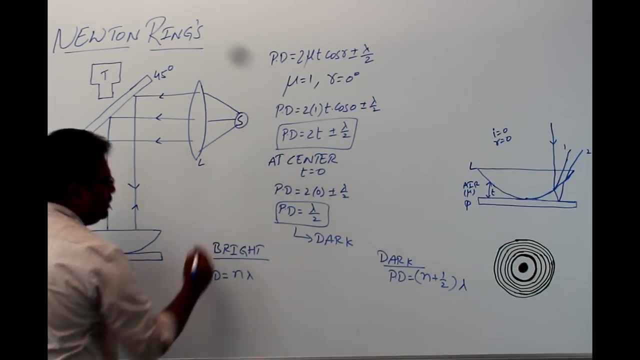 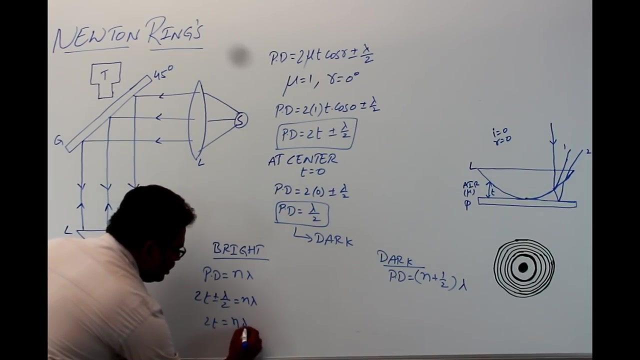 us see So, let us see, So, let us see So. Official bye, bye, bye Now. so take the path. difference here: 2t equals to 2t, plus or minus lambda by 2 is equals to n lambda. then 2t is equals to n lambda, plus or minus lambda by 2, and we can have: 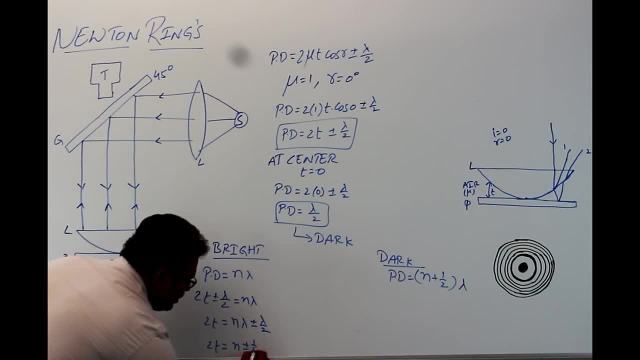 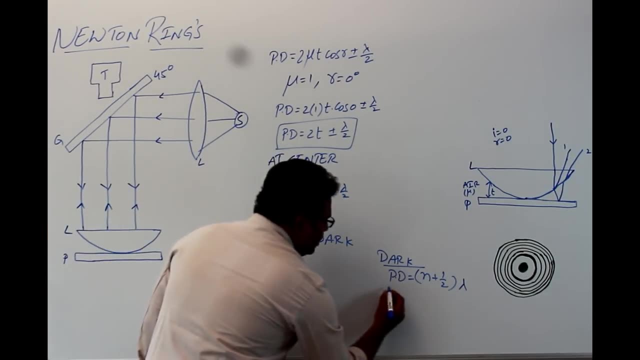 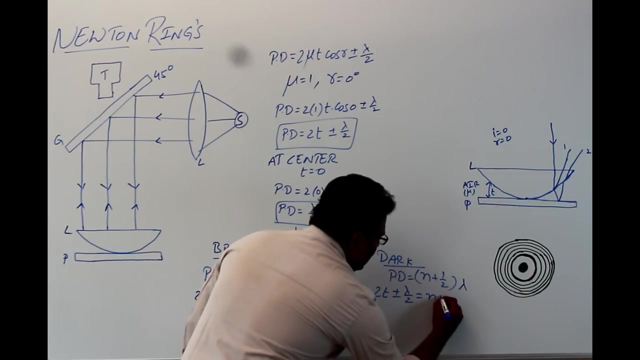 2t equals to n plus or minus 1 by 2 of lambda. So this is the condition for bright fringe under Newton's rings. and now coming here, the path difference is equals to 2t plus or minus lambda by. 2 is equals to n lambda plus. 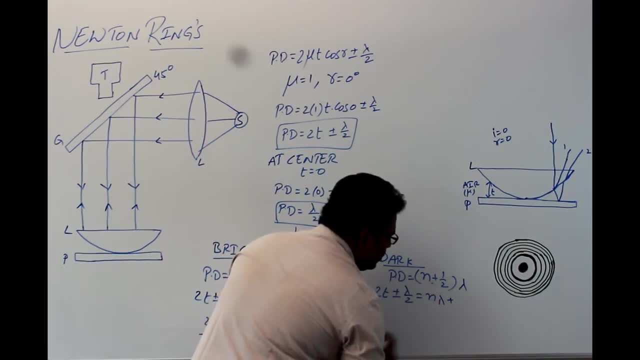 or minus, sorry, n- lambda plus lambda by 2, and if you take this plus or minus lambda by 2, that side, Then you can have: 2t is equals to 2t plus or minus lambda by 2.. So this is the condition for bright fringe under Newton's rings. 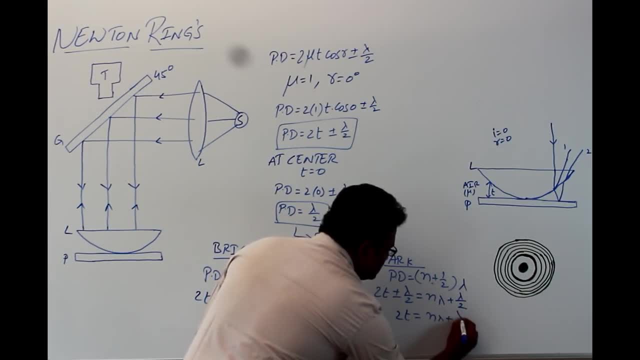 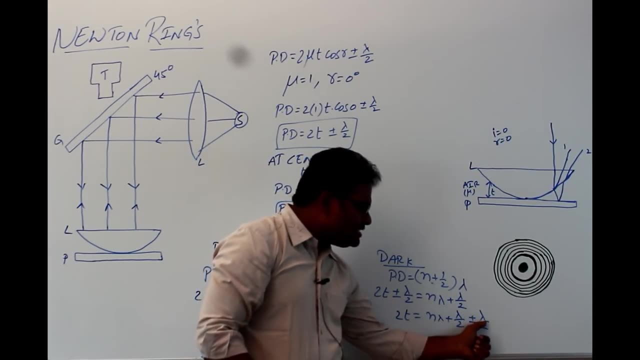 So this is delta 1, 2t via lambda zero, n is equals to n lambda plus lambda by 2, plus or minus lambda by 2.. Suppose, if you take this one lambda by 2 plus lambda by 2 or lambda by 2 minus lambda by 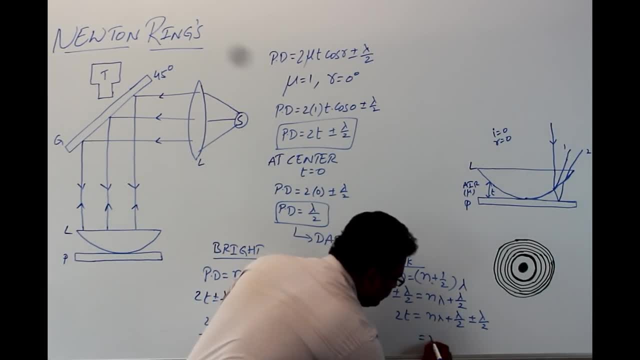 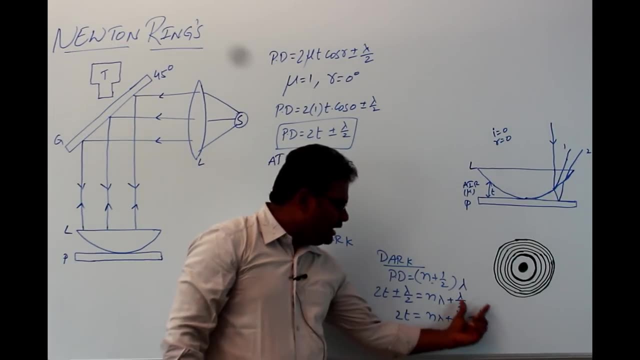 2. So will become zero. then you can have n lambda. and suppose: if it is lambda by 2 plus lambda by 2, again it will give you a lambda which is an integer. again, if you add this one to this one, you can have n lambda only. 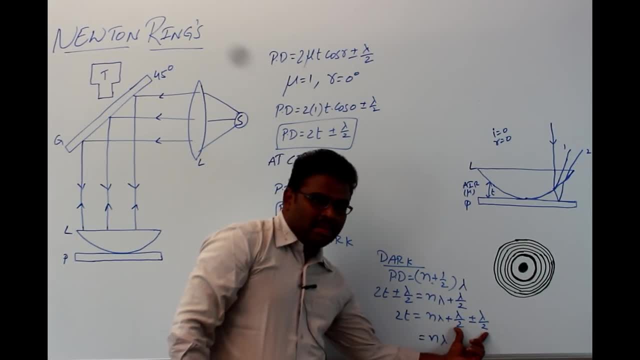 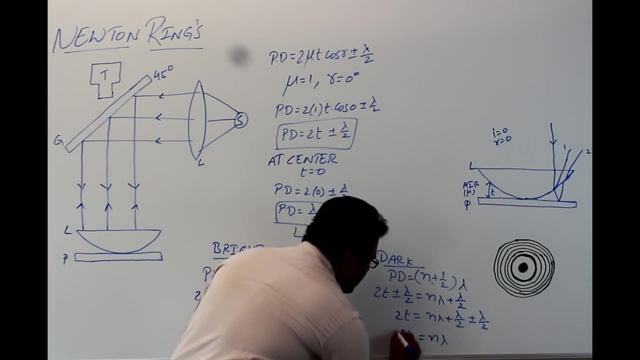 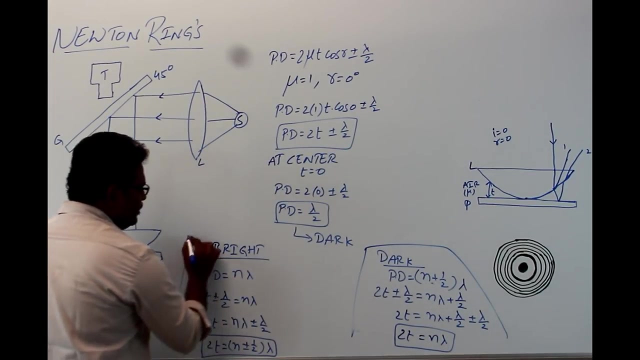 Suppose, if n is one lambda plus lambda will give you 2 lambda already. the value of 2 is there for n values. So simply we can write: 2 t is equals to n lambda. So these are the two conditions for dark fringe and this is the condition for bright fringe. So now in the next step, what we are. 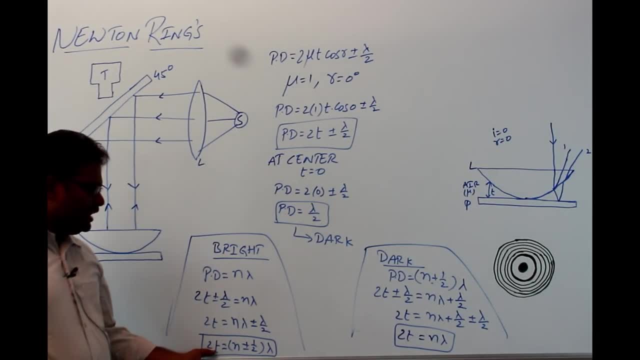 going to find out is what is the value of t and substituting value of t? one can have the diameters, since we can see the rings through the telescope, and one can calculate the diameter of the rings with the help of Bernier scales. So the condition for bright fringe is 2. t equals to n, plus or minus. 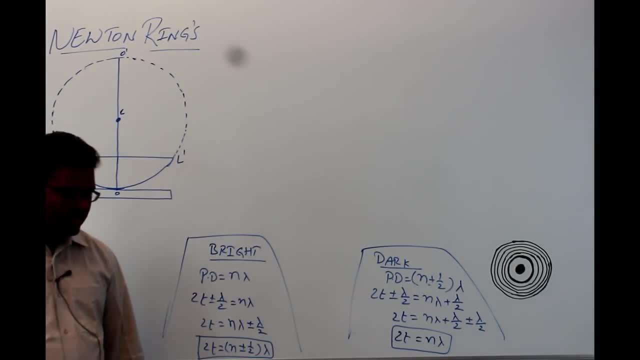 1 by 2 lambda and for dark fringe is 2. t equals to n lambda. So where t is the thickness of the AFL here. since it is a varying thickness, its center it is 0. if you keep, if you keep on moving from. 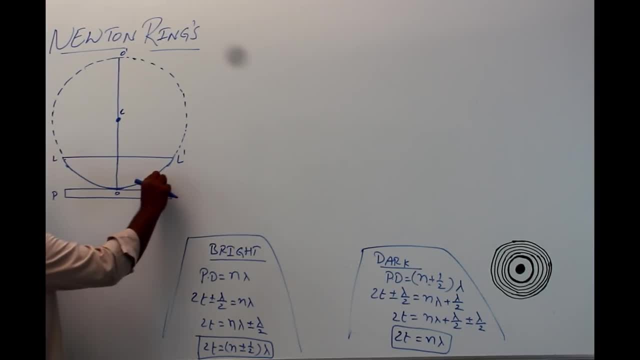 center to end point of the plan of convex lens the thickness of AFL is keep on increasing. So now to calculate for AFL, Take a plan of convex lens on a plate P and extend the surface of plan of convex lens. then you can have the radius of curvature of this plan of convex lens. let us say capital R. and now, at certain 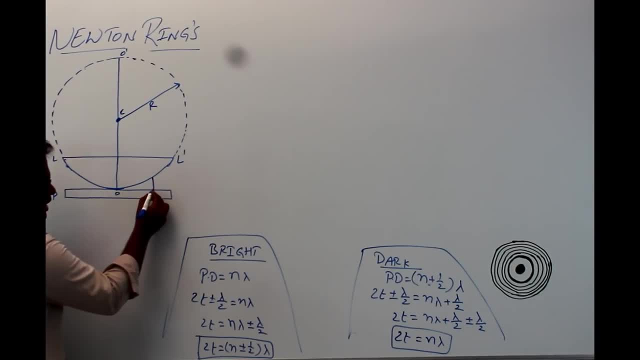 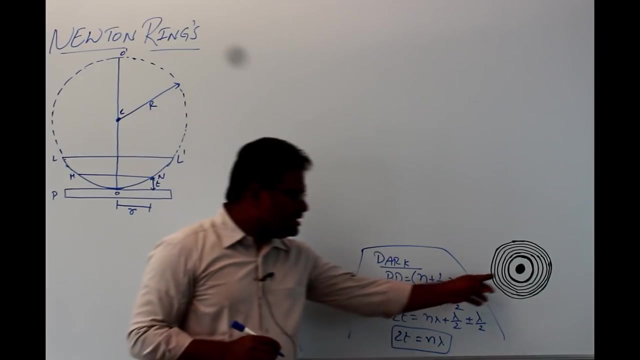 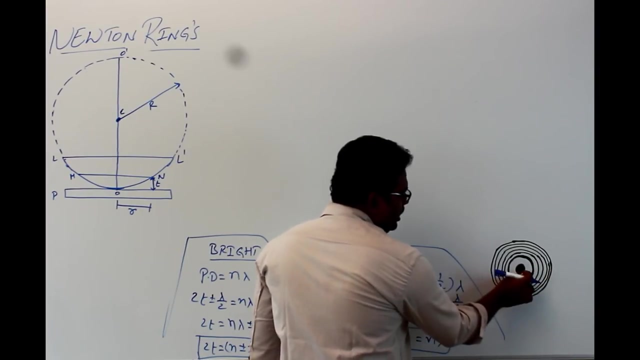 thickness, at certain height or at certain thickness: T, take a ring of radius, take a ring m and n of radius, small r. So at center- already we discussed the center- we are having a dark range and then and then you can have bright, dark, bright, dark, bright. and now, 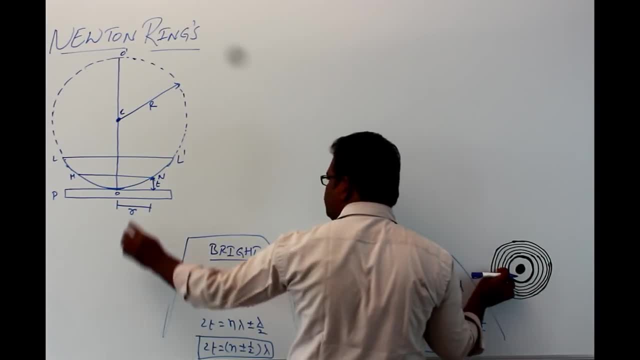 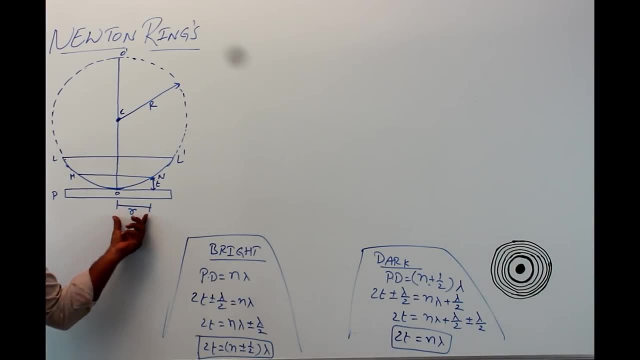 some. take some ring here, at this position, at a height T. take something that way, be bright or dark. take some ring of radius, small r. and now let us call this interacting point as Q, since the value of Qo is T and the value of oo is 2r, since from center to here the radius of curvature is R. from here to here is R the total. 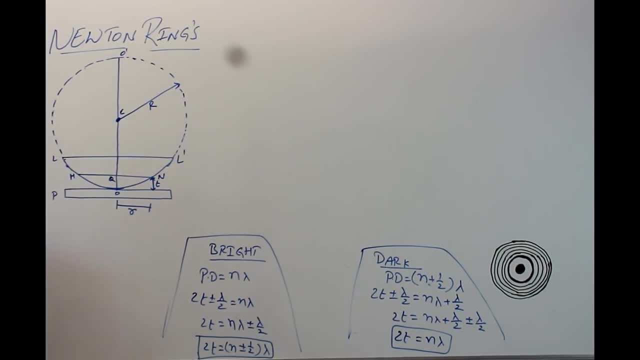 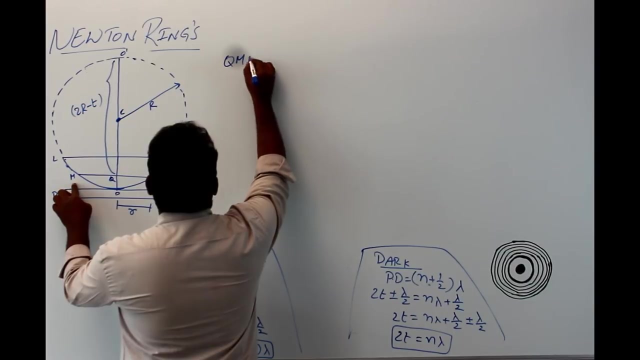 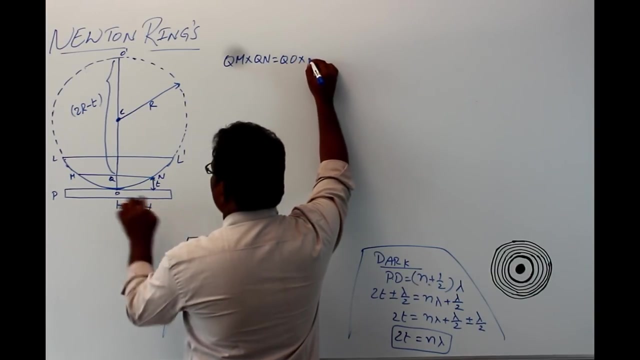 value of O is 2r and the value of Q is t, then the value of Q will become 2r-t. from the symmetry or the, from the law of circles we can have, from the geometry of circles, one can write QM into QN is equals to QO, into QO, dash, nothing but. 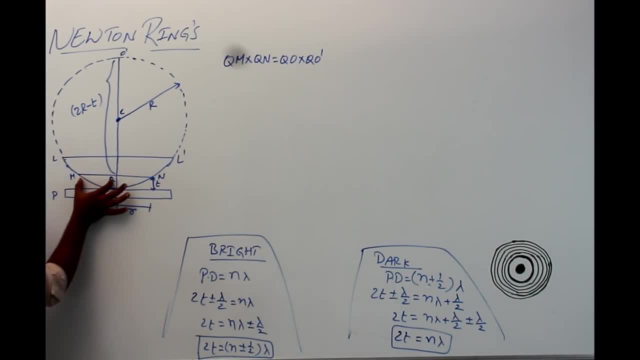 the products of the chords are equal, like MQ into QN is equals to QO into QO, dash, since they are not equal, but their products are equal. one has to remember that. and now the value of MQ and QN: since MN is a ring, their radius also equal, so the 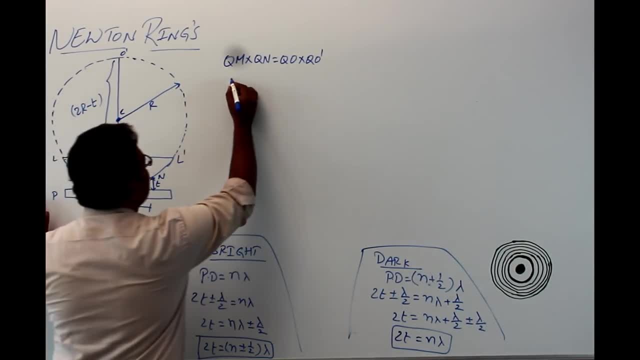 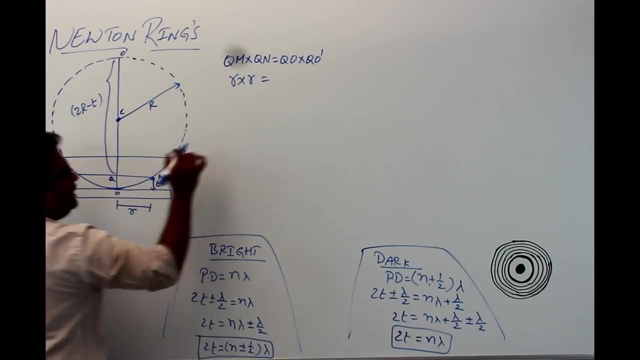 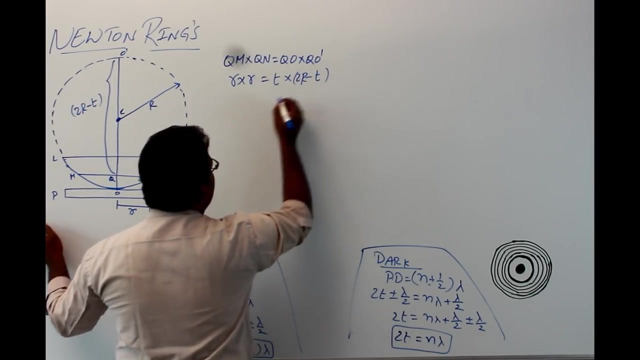 value of QN is R and MQ is also R, so one can write R into R. that's equals to the value of QO. the value of QO is t into the QO dash is 2r-t. then if you multiply then you can have R square equals to 2rt-t square, since 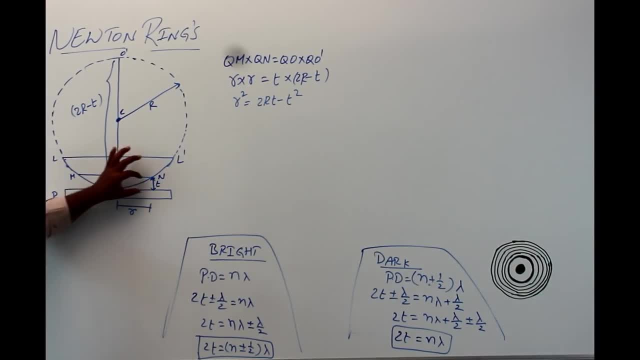 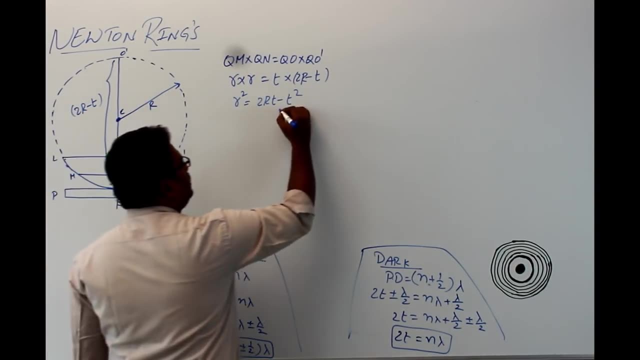 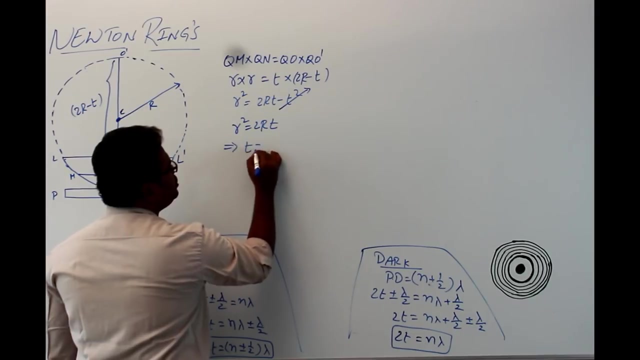 p is the thickness, which is very thin or it's a thin film. so if you square the thickness, t can have very small value. so one can neglect the value of t-square. then you can have R square equals to 2R x t. that implies t equals to R square. 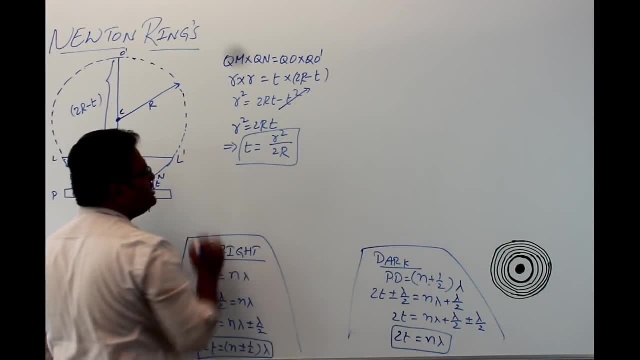 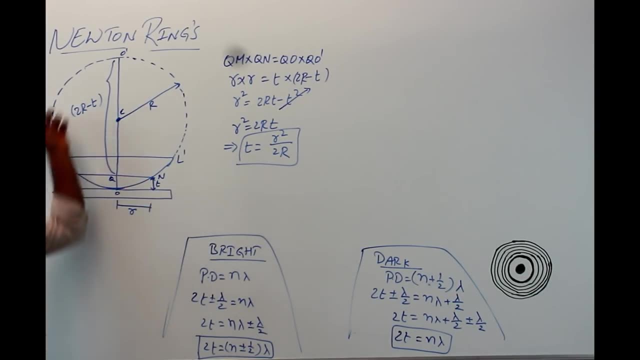 by 2R, where smaller is the radius of the ring- that may be bright ring or the dark ring- and capital is the radius. R is the radius of青QN. so then go back to this edge and multiply: R is 2R of curvature and t is the thickness of that particular ring. 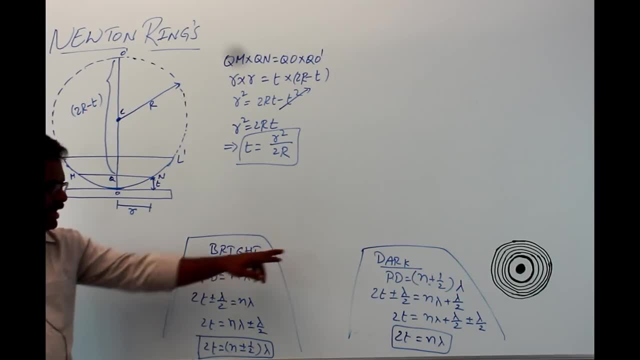 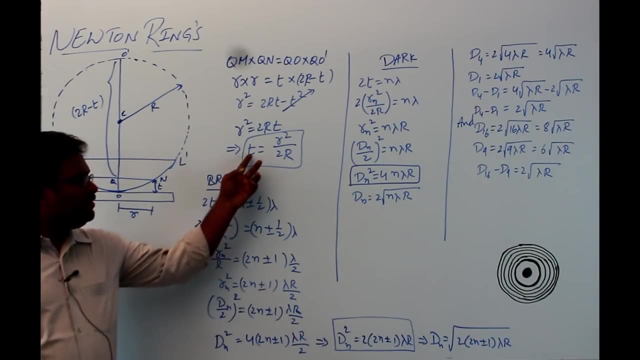 So now take the value of t and substitute the conditions in bright and dark conditions. So take the condition of bright fringe: 2t equals to n plus r minus 1 by 2 lambda and substitute the value of t, r square, by 2r in this condition. 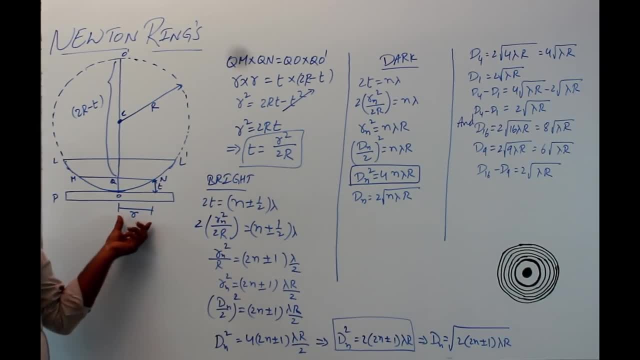 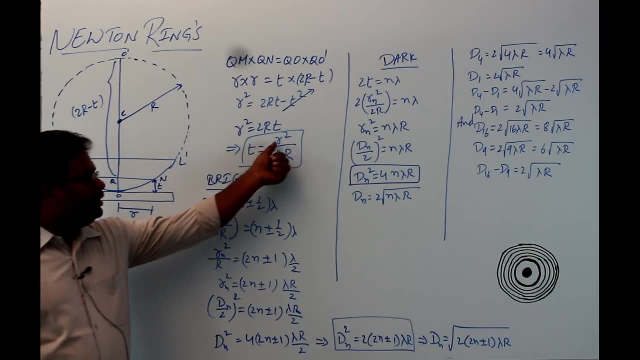 Since r is the radius of a particular ring. suppose if it is fourth ring, fourth ring radius. fourth bright ring. fourth bright ring radius. sixth dark ring, dark ring radius. So now take the value and substitute. in this condition, t equals to rn square, since n stands. 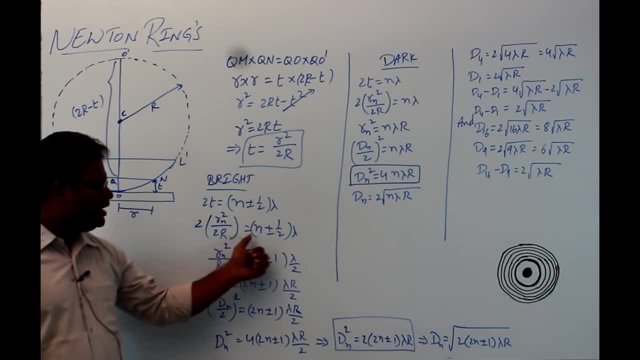 for that particular ring number and rn square by 2r equals to n plus r minus 1 by 2- lambda. And if you solve this, one rn square and everything get cancelled. 2, 2 get cancelled. rn square by r equals to 2n plus r minus lambda by 2 and rn square equals to 2n plus r minus 1. 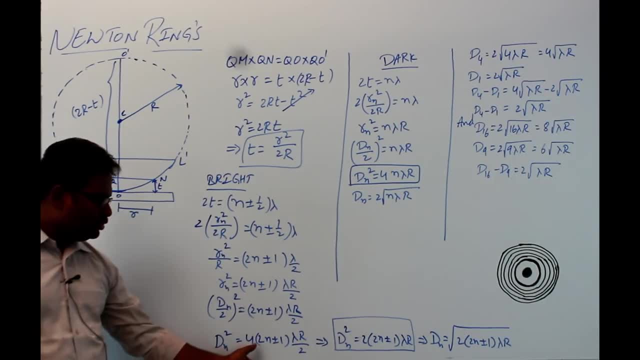 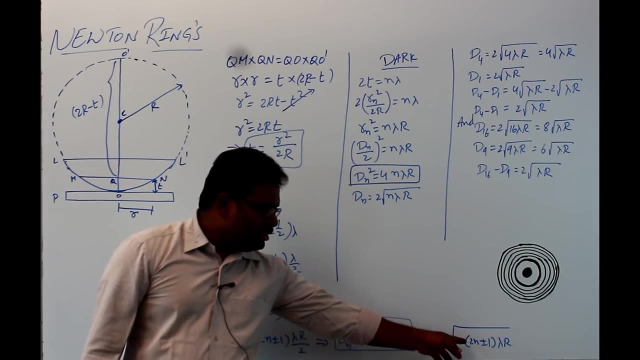 lambda r by 2, and finally you can have dn square equals to 2 of 2n plus r minus 1 lambda by r, And that implies dn equals to 2n- 2n, 2 of 2n plus r minus 1 of lambda r. since this is, 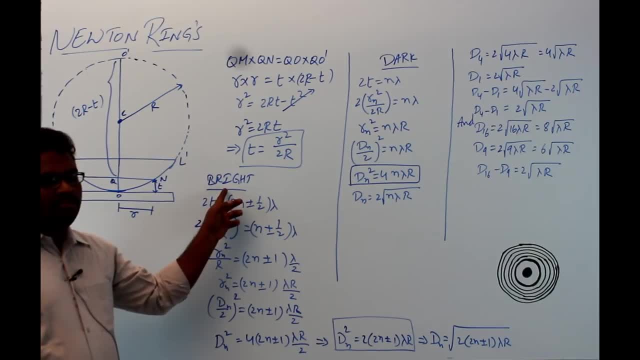 the diameter expression for bright ring. Why we are so concerned about diameter means we can see literally through the telescope which is kept on the top of the glass plate. And finally, if you take the condition for dark ring, 2t equals to n lambda, and by substituting: 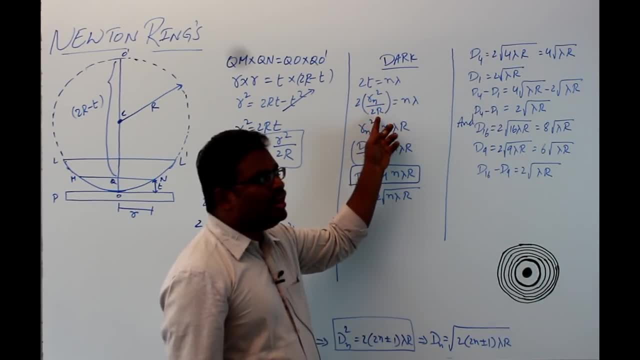 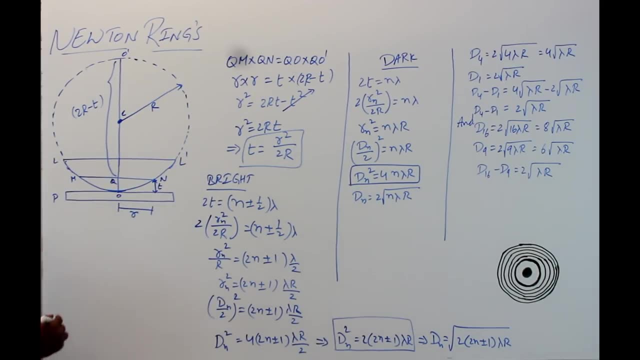 the value of t in this particular one, rn square equals to 2r, since rn is the diameter, sorry radius, of that particular dark ring And And one can write that rn diameter, rn square. we know that diameter equals to 2 of the radius. 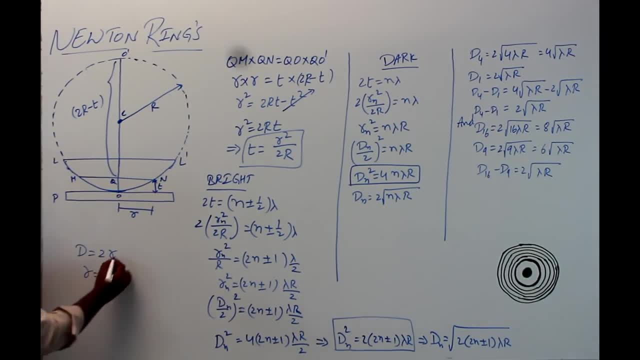 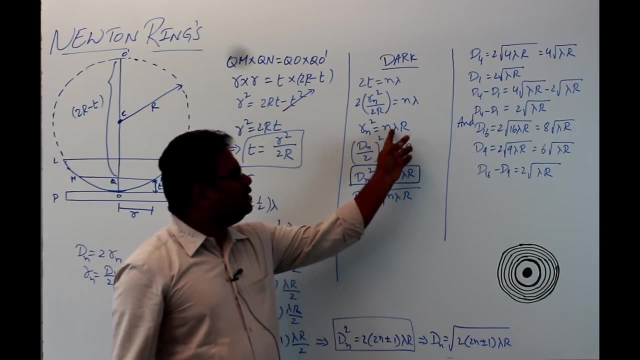 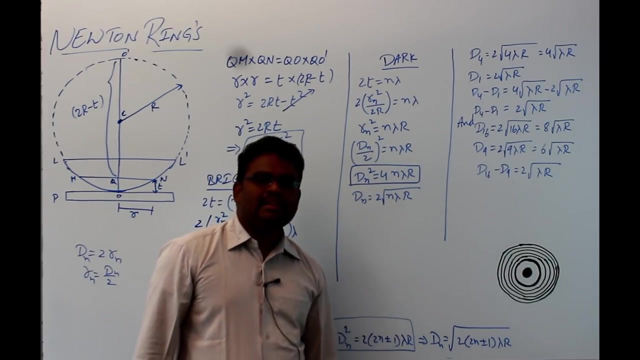 and then r equals to d by 2.. If rn is a particular ring radius, then dn will become its diameter. Then rn square is equals to n lambda r. finally, you can have dn square equals to 4n lambda r. So by using the expressions one can calculate the diameter of bright rings and dark rings. 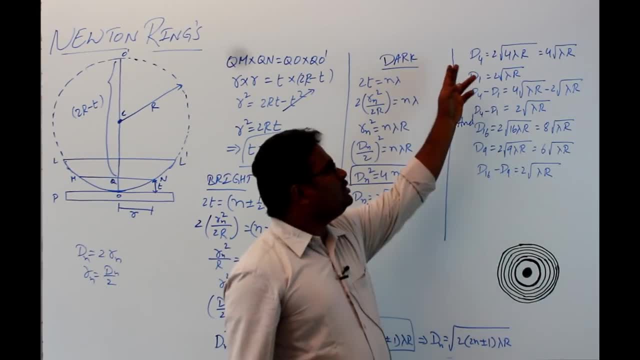 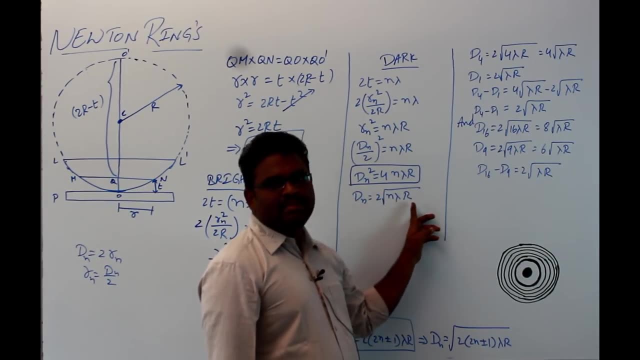 And next, If you take d4, so that means diameter of 4th dark ring, the expression for dark ring is: dn, equals to 2 under root n lambda r, and if it is for 4th ring, n value is 4.. 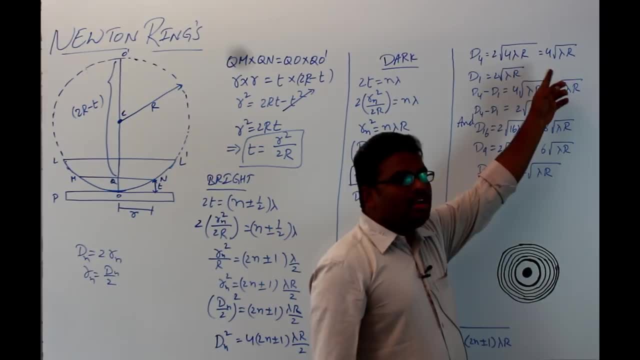 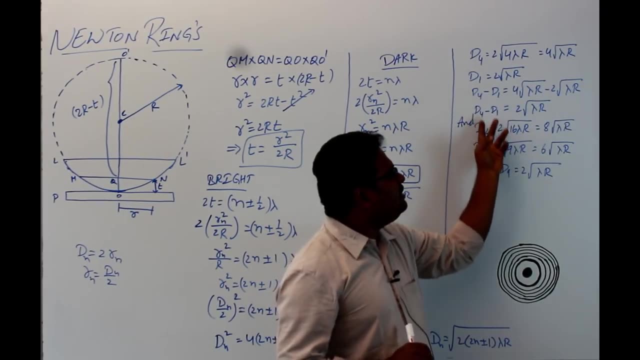 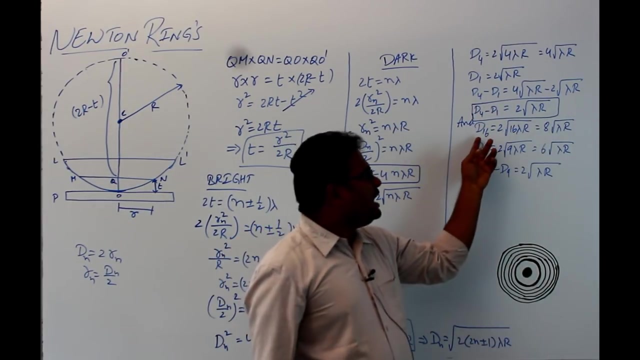 So 4 lambda r, then you can have 4 under root lambda r, and for d1, first dark ring, it will be 2 under root lambda r. d4 minus d1 will give you 2 of under root lambda r. Similarly, if you calculate for 16th dark ring and 9th dark ring, then also you can have d16. 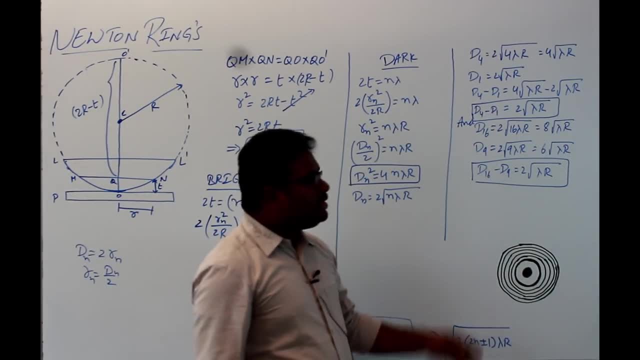 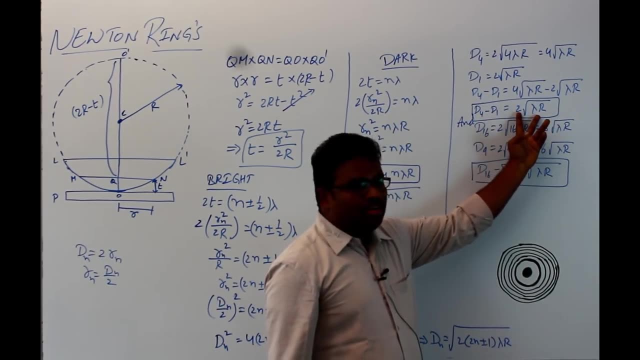 minus d9 as 2 root lambda r. So if you particularly observe these two expressions, in between 1st and 4th ring the value is 2 root under lambda r. In between 9th and 16th ring also, the value is 2 root lambda r. 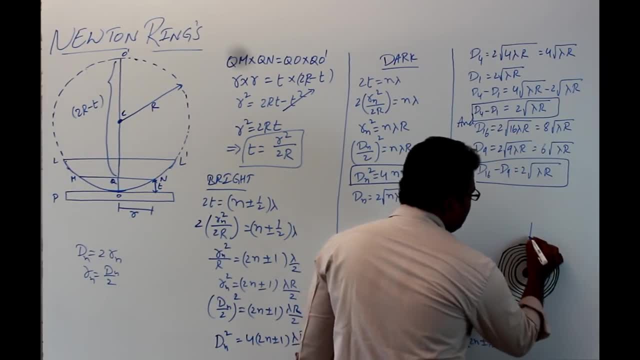 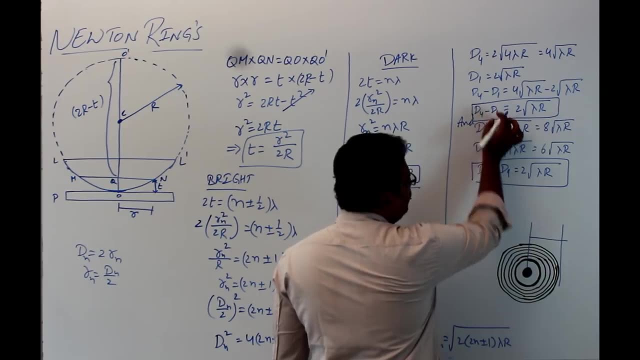 So if you keep on moving from center to end part of the rings at the center we are having within a gap of 4 to 1.. Suppose 4 to 1 you have the value is 2, root lambda r only the gap between 4th dark ring. 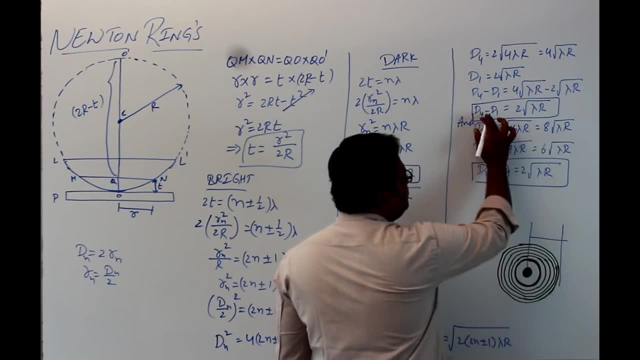 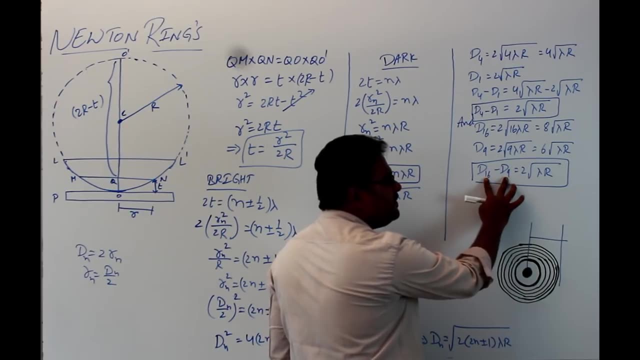 and 1st dark ring is 2 root lambda r, And that means there is a span of 3 rings only, But if you consider 9 and 16, there is around 7 rings, even 7 rings also spaced in a gap. 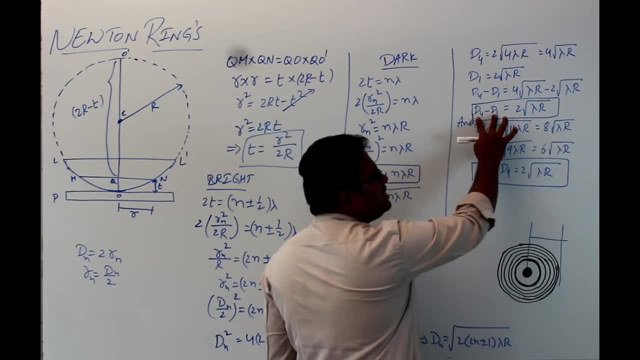 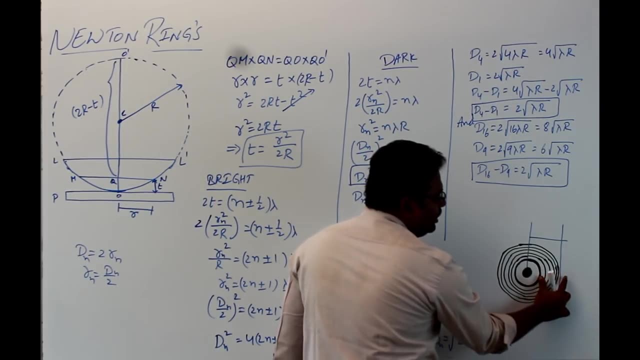 of 2 root lambda r. Here the 3 rings are spaced in a gap of 2 root lambda r. That means if you keep on moving from center to end part of this one, the closeness will be decreased. The distance between 2 rings will be decreased. 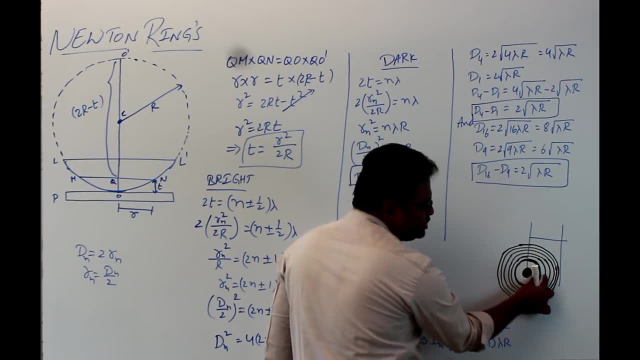 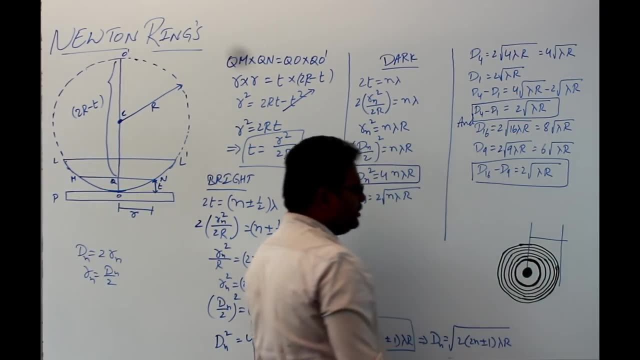 Initially. if you observe that one, the gap between the 2 rings is very less. if you keep on it's high and if you keep on moving, the gap between the 2 will be come closer to each other. So this is about why the rings are closely spaced. 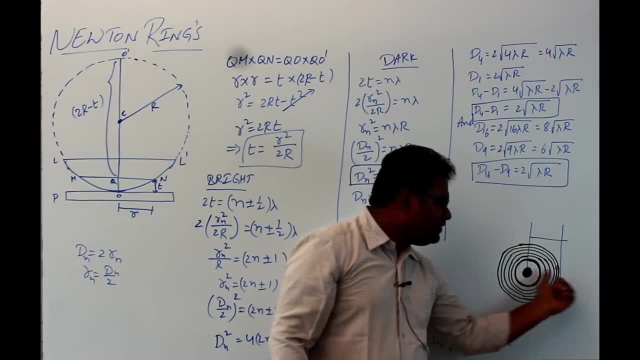 Now, if you keep on moving from center to end, the gap between the 2 rings will be come closer to each other. It will be spaced if you keep on moving from center to end part. So this is the reason within a gap of 2 rings. also, you have the same value within 3 rings. 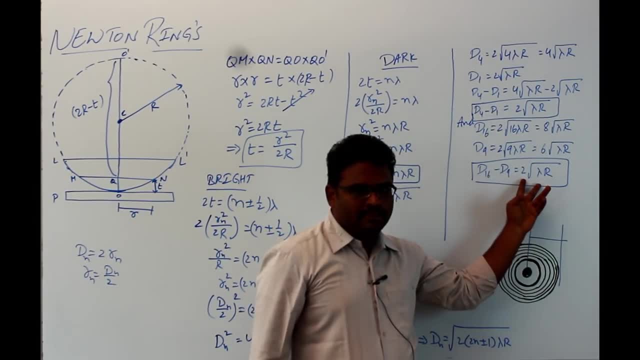 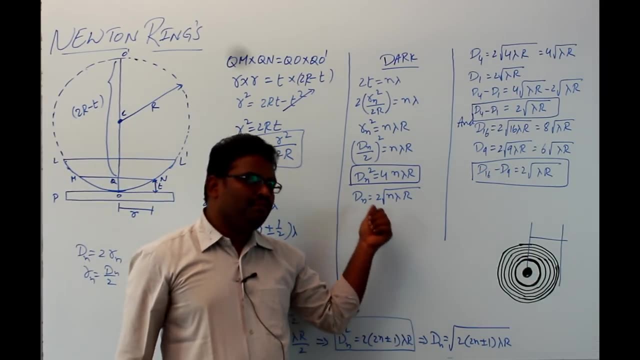 also, you have the same value. within a gap of 7 rings, also, you have the same value. So this is about Newton's rings. And next step, what we are going to see is: how can we find out the radius of curvature? if you don't know r, how can we calculate? and if you don't know lambda, how can we calculate? 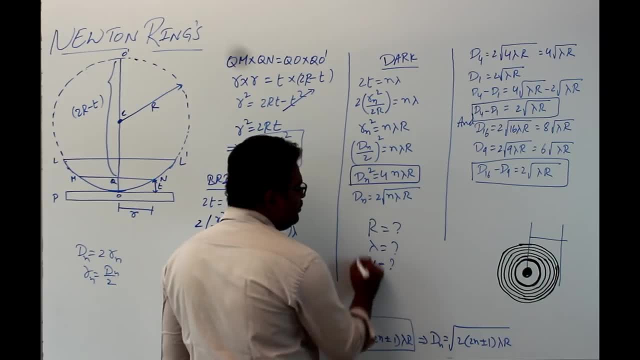 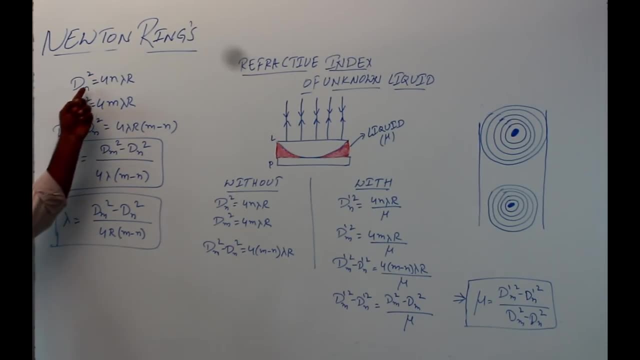 and if you don't know, mu refractive index of an unknown liquid, how can we calculate? We can see in the next lecture, Thank you. next step: As we already calculated, the diameter of dot ring dn square equals to 4m. lambda r for: 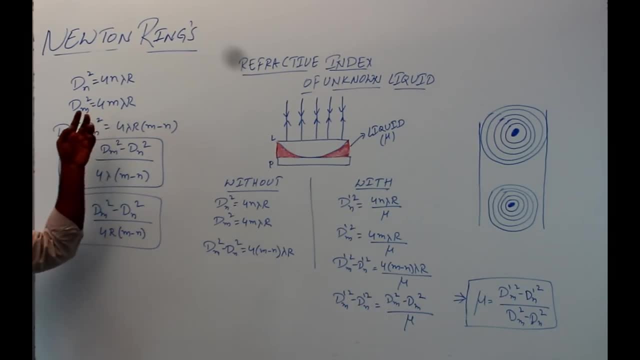 a particular ring number, n, and for a particular ring number, m, dm square can be written as 4m lambda r. So now dm square minus dn square will give you 4 lambda r of m minus n and by. if we want to know the unknown radius, curve, curvature of a given plan of convex lens, then take a known 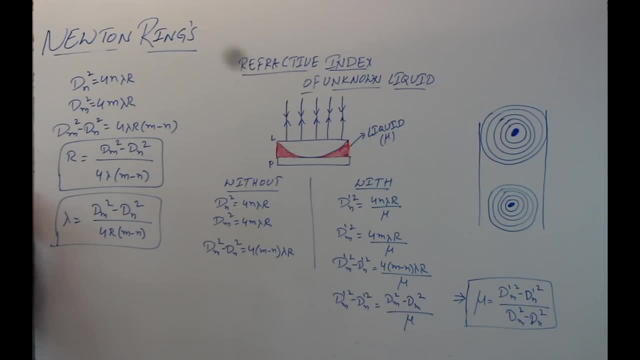 lambda value of a monochromatic source of light whose wavelength and whose wavelength is around. if it is sodium vapor lamp it is 5893 angstrom units Like that. take the known value of lambda, then we can find out the r of unknown value. Suppose. if you want to know the unknown value, 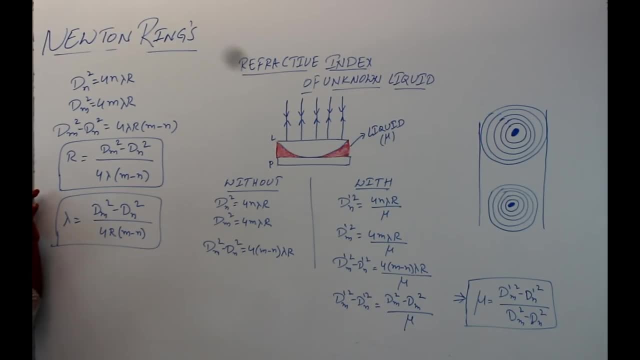 of wavelength or lambda of a given monochromatic source of light. then take a known plan of convex lens, of radius of curvature r, and with the help of telescope one can find out the diameter of m3.. And then the dot rings. So by using these two expressions one can calculate the radius of. 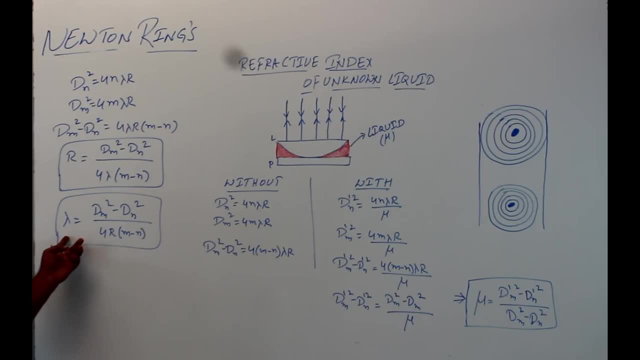 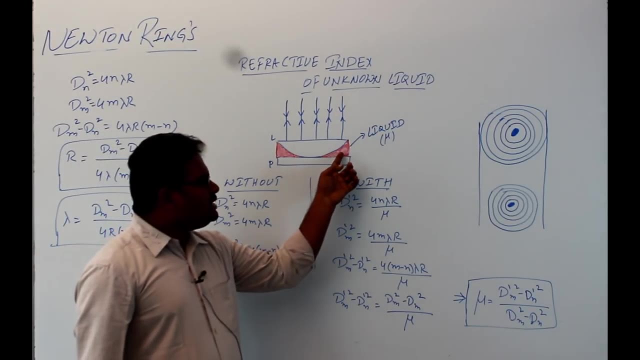 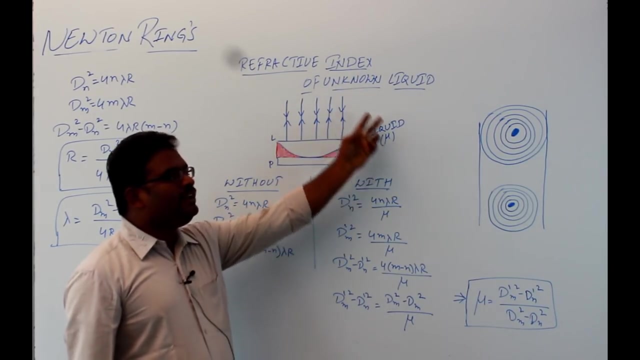 curvature of lenses and wavelength of unknown sources. and also we can calculate the refractive index of unknown liquids. How can we calculate? Let us see, Since the air film is, since the thin film is occupied by air previously, suppose, if I want to calculate the refractive index of an 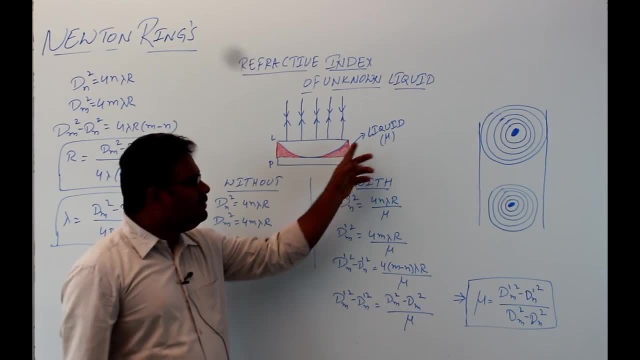 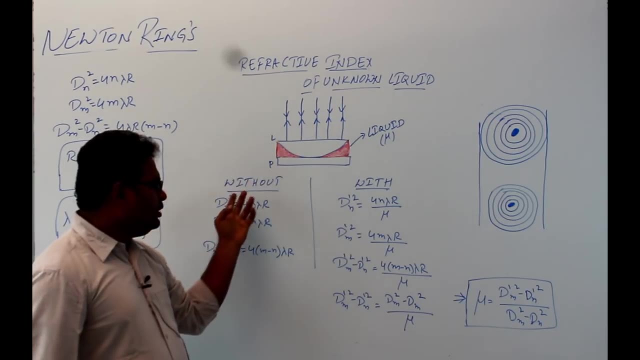 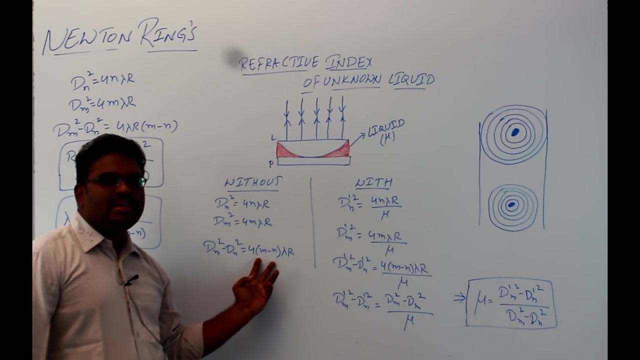 unknown liquid. fill the air column or the thin film with that liquid of refractive index mu. So first do the experiment as like previously, then without this liquid, then you can have a dn square minus dm. square minus dn square equals to 4 m minus n of lambda r. Now keep the liquid and do the. 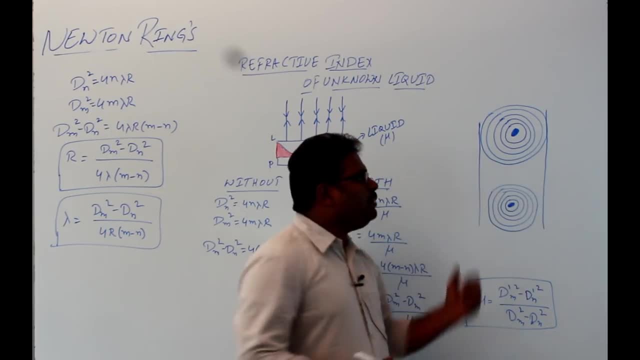 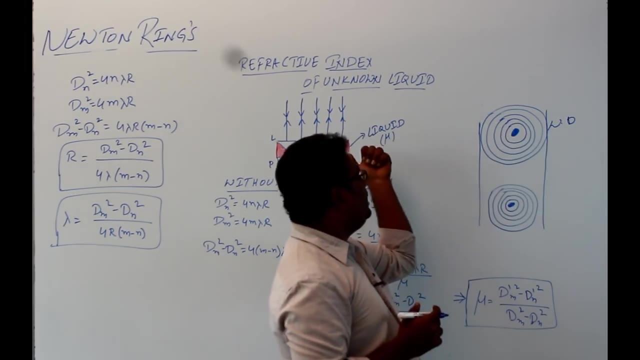 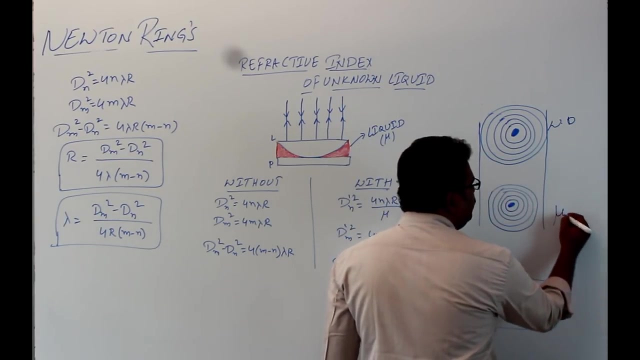 experiment, What the thing that we can found is without liquid. without liquid, if you get the rings diameters like this by keeping the liquid in the film- part thin, film, part Umm- the diameter of the rings will decrease by an amount of mu, Decrease the size or the diameter. 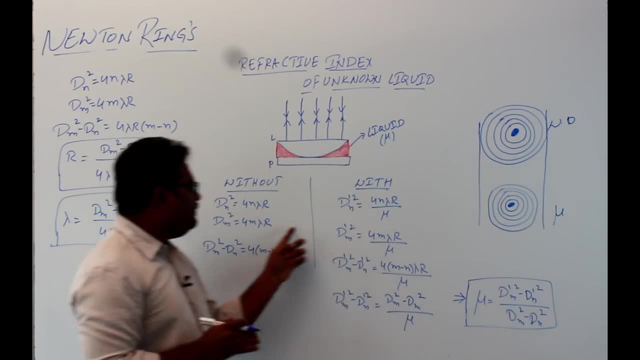 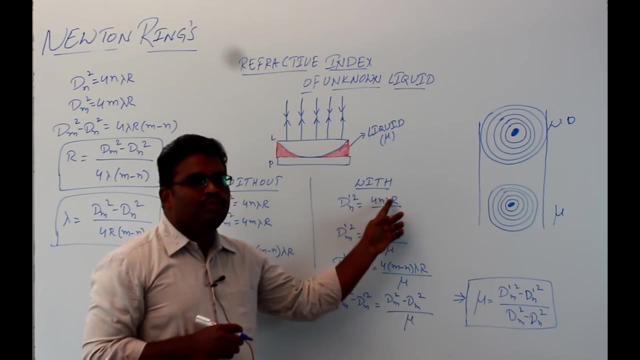 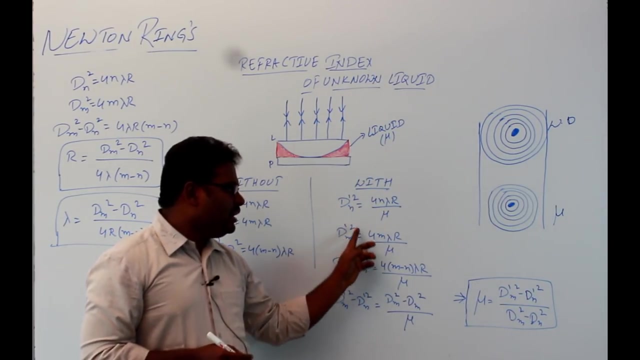 of rings will decrease. So if it decrease initially without liquid, if it is dn square equals to 4n lambda r, with the liquid it will become dn dash square equals to 4n lambda r by mu, where mu is the refractory index of this one. And now for a particular M3, dm dash square is: 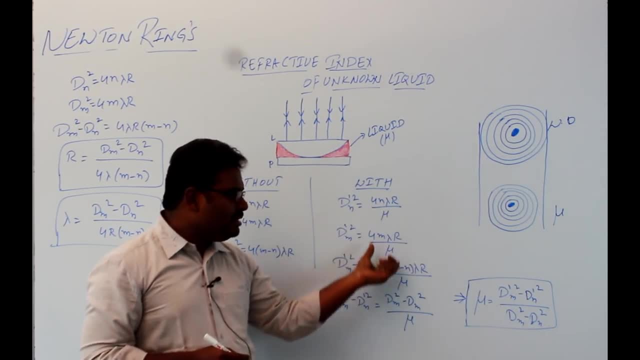 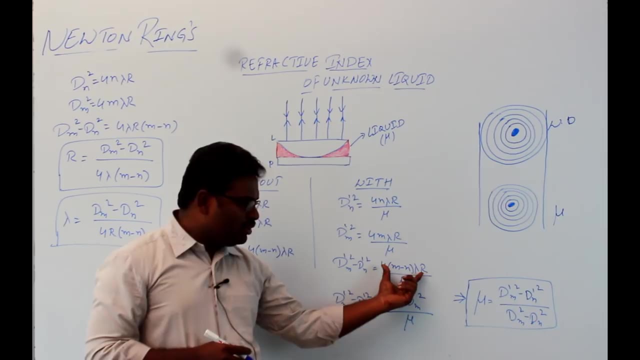 equals to 4m lambda r by mu. So since the diameters are decreasing and dm dash square minus dn dash square equals to 4m minus n lambda r by mu, since 4m minus n lambda r is nothing but dm square minus dn square and substitute here, then you can have this expression: 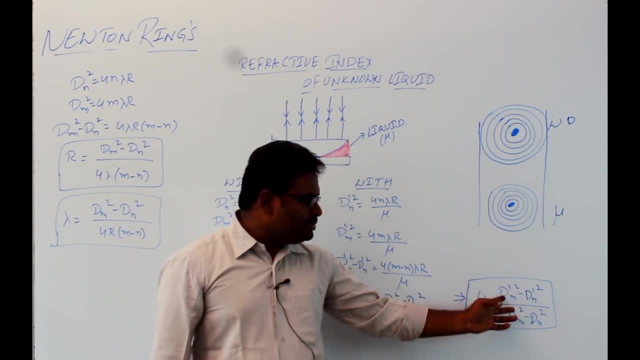 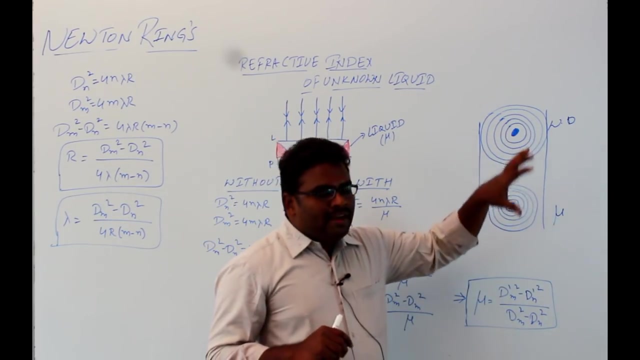 From this one can calculate: mu equals to dm dash square minus dn dash square by dm square minus dn square. So with the help of this equation one can find out the refractory index of unknown liquids. And one has to remember: in reflected case only this is In reflected case. 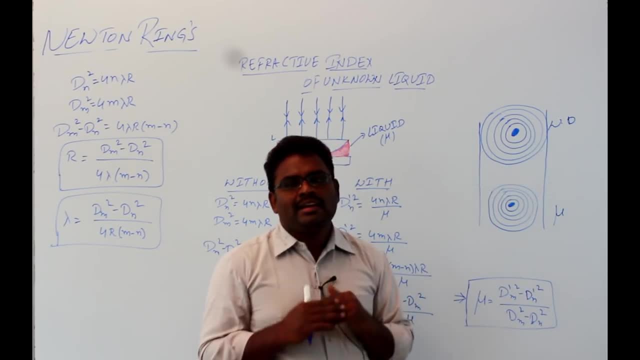 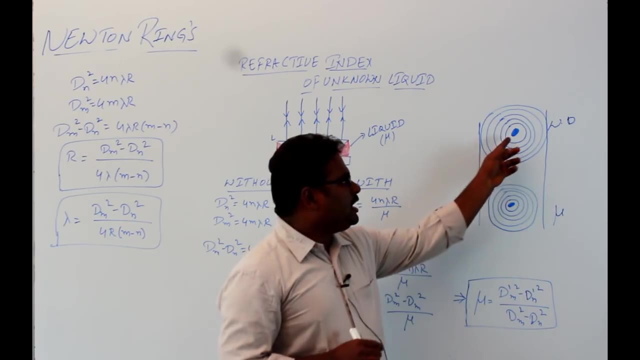 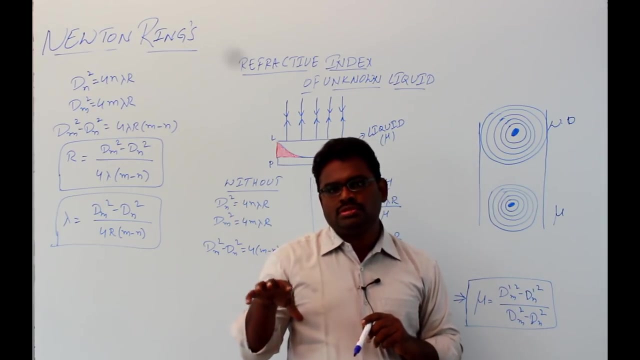 the center spot is dark and in refracted case, if you see the Newton's rings from the bottom of the glass plate P, then you can have a bright range. And now the color of bright also depend on the type of monochromatic source of light that we are using. If we are using a yellow color source, 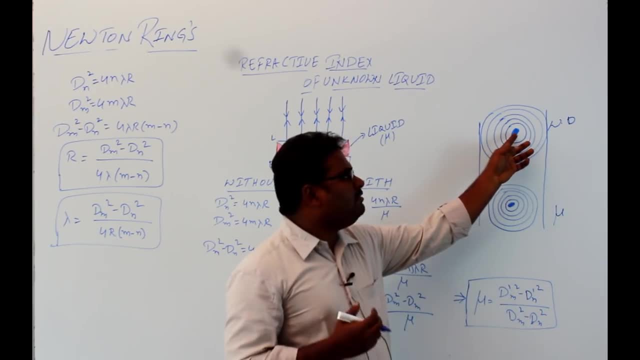 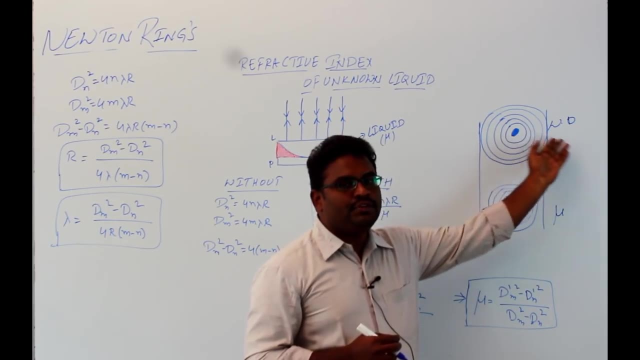 then the bright will be yellow color. So then the pattern will be like this: dark Yellow, dark yellow, dark yellow Of decreasing. all the rings will come closer if you move from center to far away. So this is about Newton's rings. 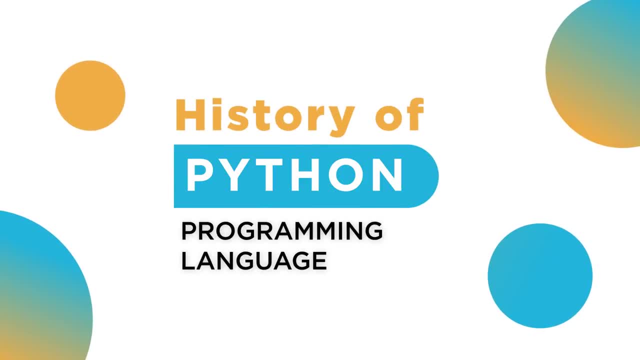 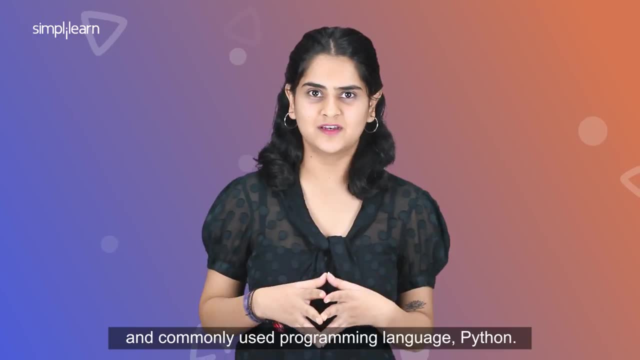 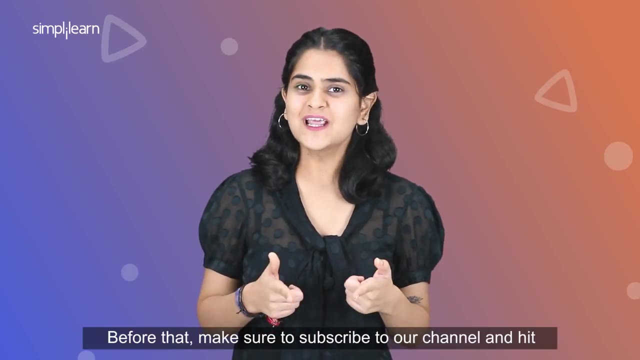 Hey everyone, in this week's episode we'll talk about the most popular and commonly used programming language, Python. So let's begin and learn about the development of Python and gain insights about the current IT trends. But before that, make sure to subscribe to.